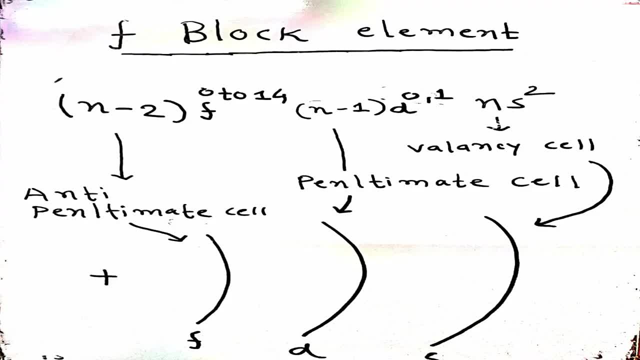 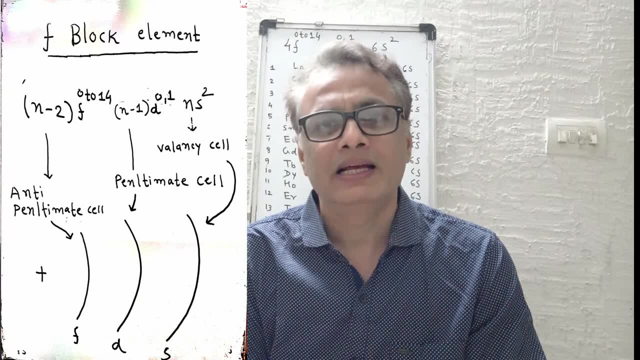 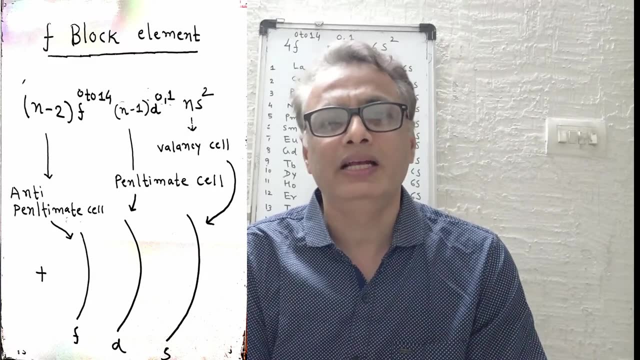 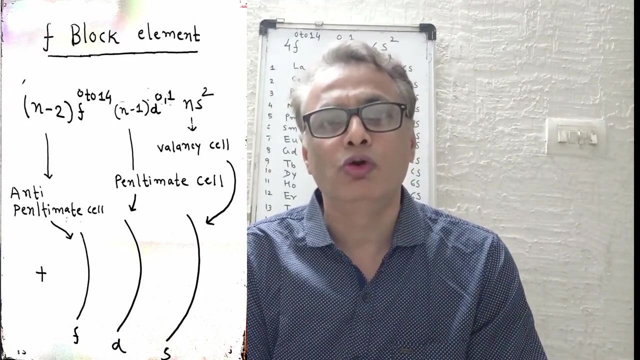 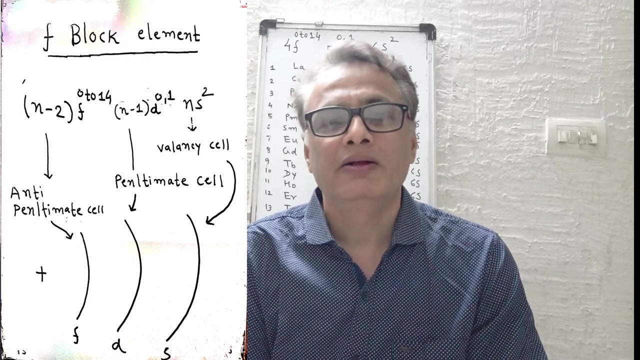 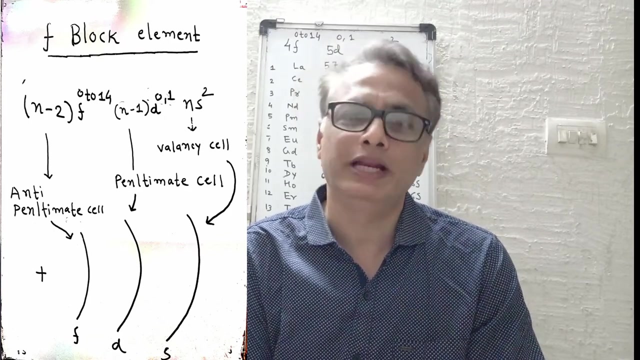 contain two electron. Before valence cell, D orbital is there, that is known as penultimate cell, which may contain 0 or 1 electron, and N-2F0214 are known as antepenultimate cell, which is known as F orbital, which may contain 1-14 electrons. F block element. 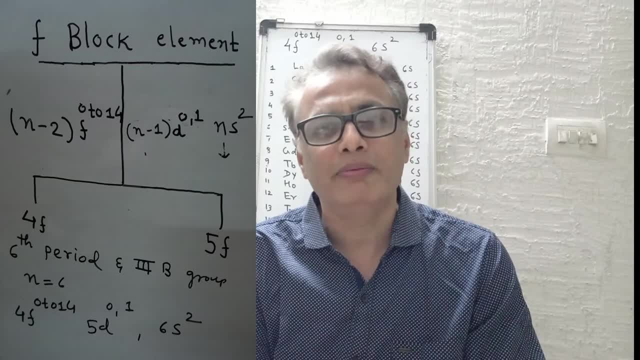 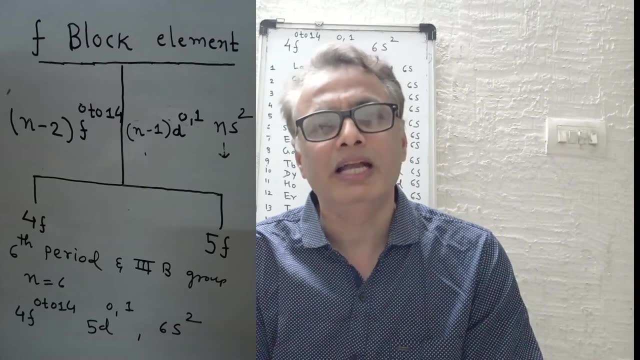 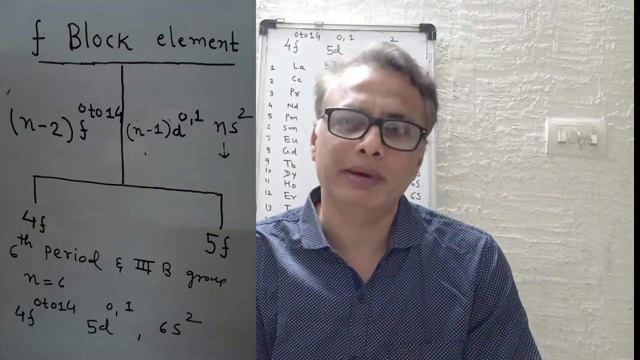 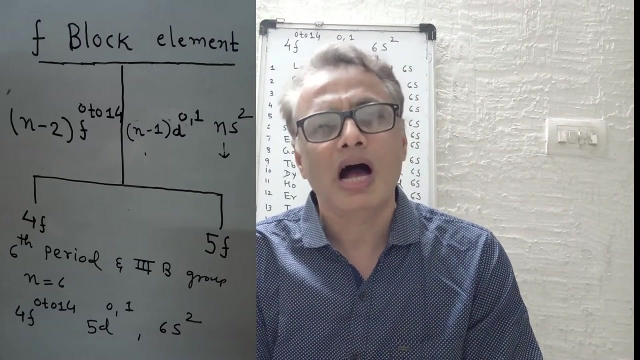 can be classified into two different type: 4F block element and 5F block element. 4F block element is defined as the element in which new entering electron takes position in 4F orbital. are known as 4F block element. The element in which new entering electron takes position in 4F orbital are known as. 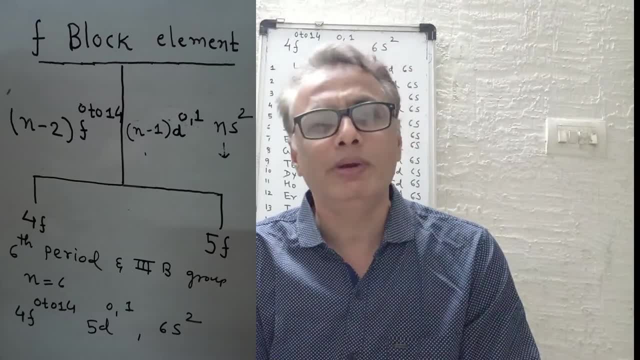 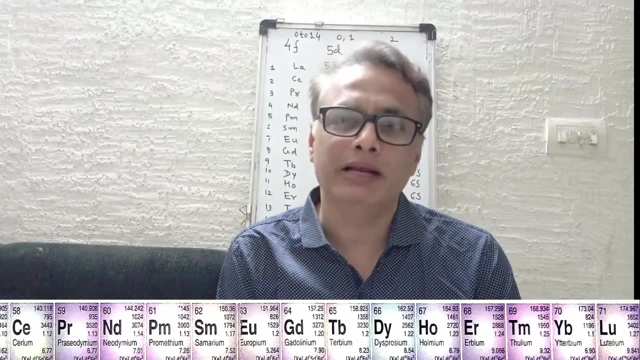 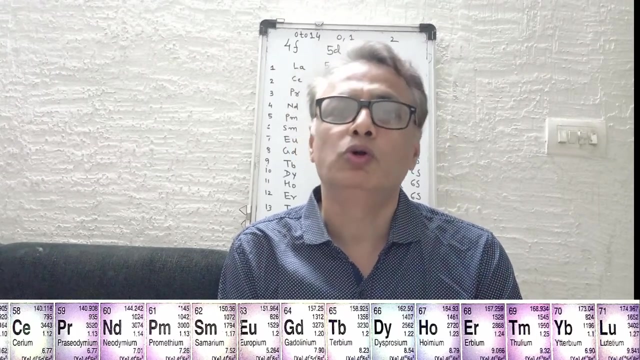 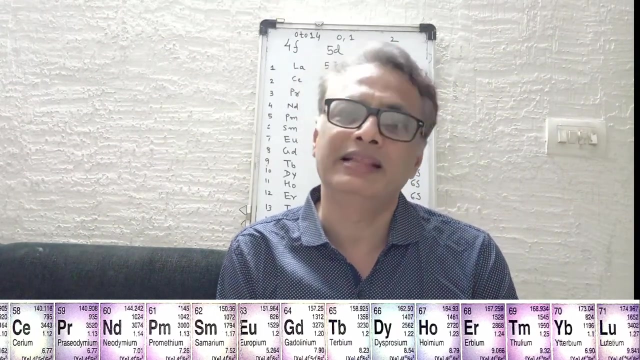 4F block element. Atomic number 58 to 71 are known as 4F block element, or we can say that elements starting from cerium to lutetium are known as 4F block element, which are also known as lanthanide elements. 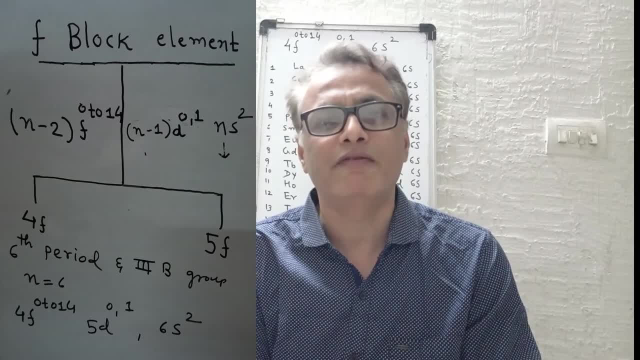 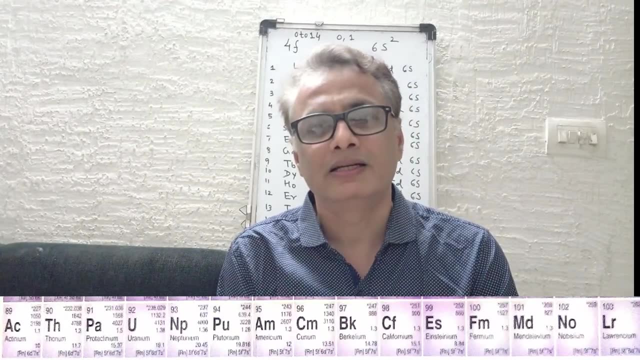 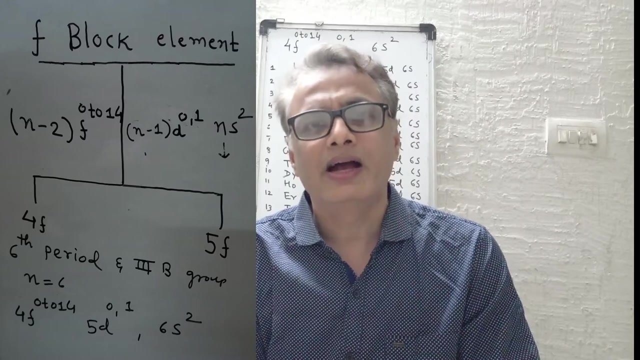 The element in which new entering electron takes position in 5F orbital are known as 5F block element or actinides element. Lanthanide elements comes under 6th period and 3rd B group in periodic table. Lanthanide elements comes under 6th period and 3rd B group in periodic table. 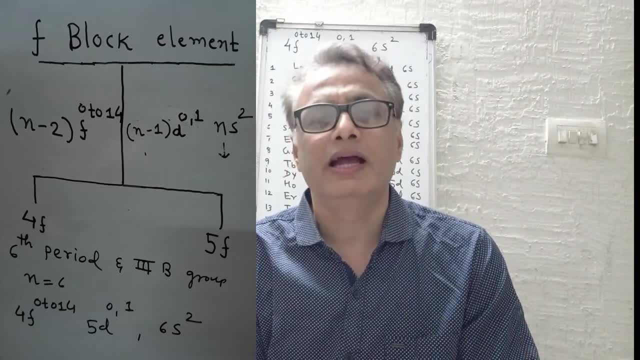 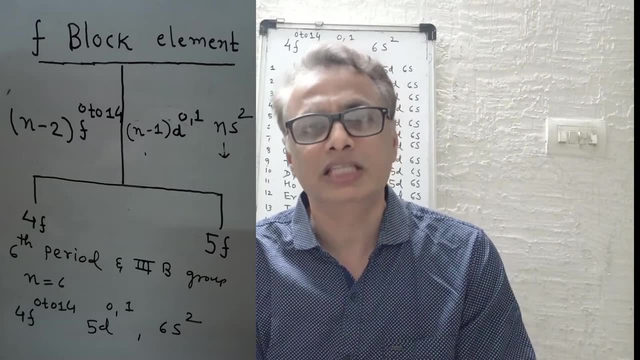 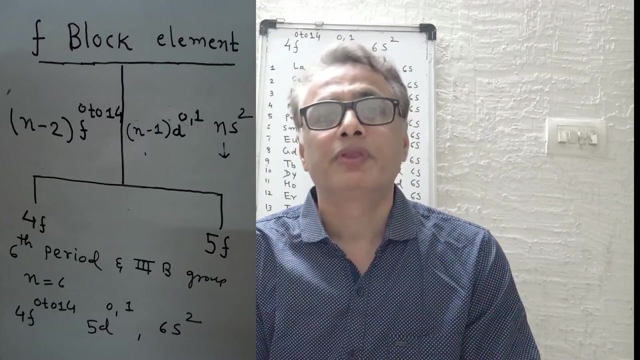 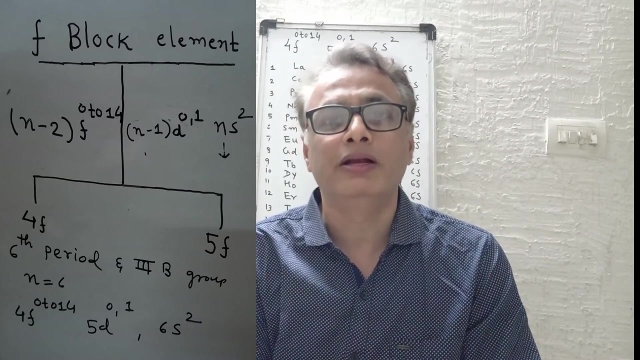 and third B group in periodic table and general electronic configuration of lengthened element can be written here. it comes under sixth period. therefore we will take N is equal to 6 and substituting the value of 6 in general electronic configuration of F block element, that is N minus 2 F, 0 to 14 N. 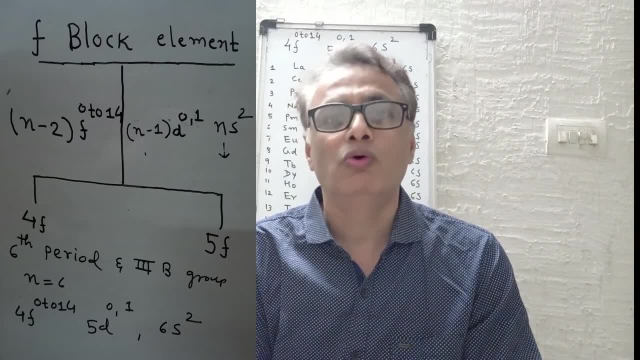 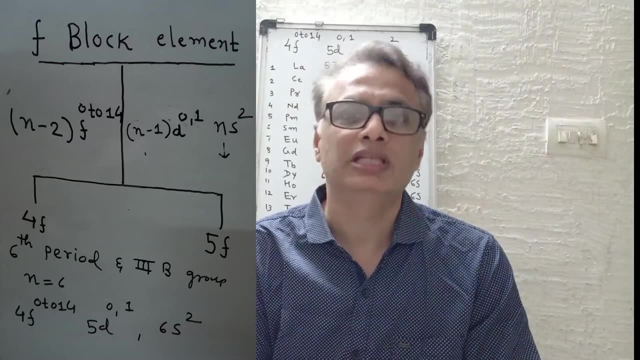 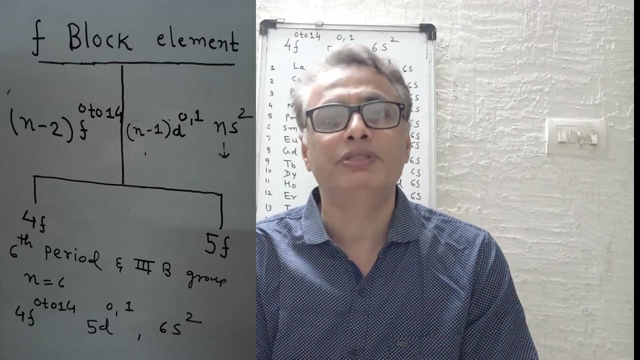 minus 1 B, 0, 1 N, s, 2, we would get 4 F 0 to 14, 5 D 0, 1, 6 s, 2. this is general electronic configuration of lengthened element. so general electronic configuration of lengthened element can be written: 4 F 0 to 14, 5 D, 1, 6 s, 2, and it is: 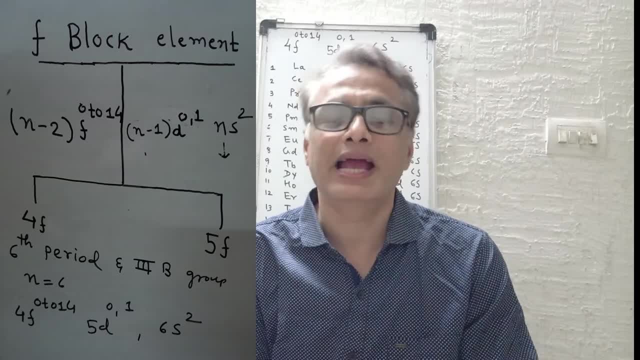 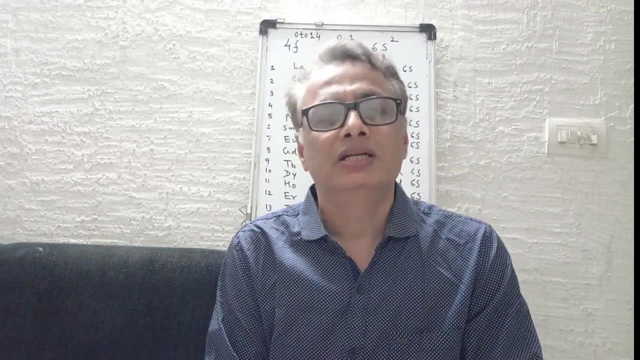 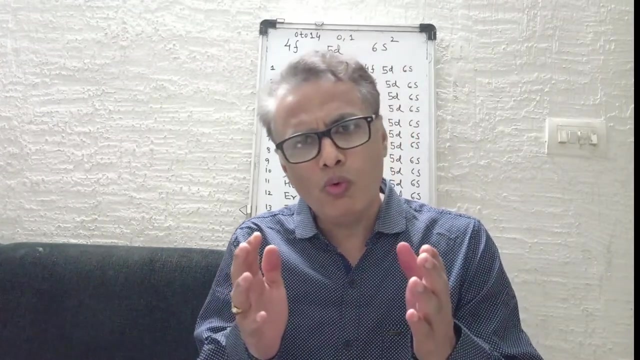 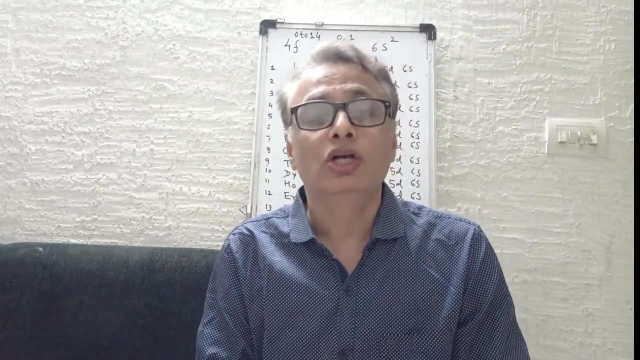 denoted by ln symbol. it is denoted by ln symbol. now we are going to write name symbol, atomic number and electronic configuration of length in an element. you have studied name symbol, atomic number and electronic configuration in 12th standard, so I am going to give you. 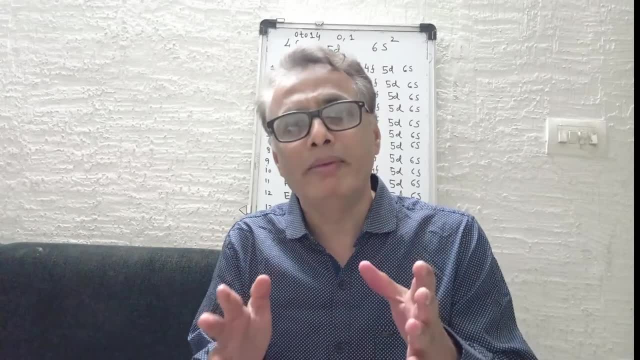 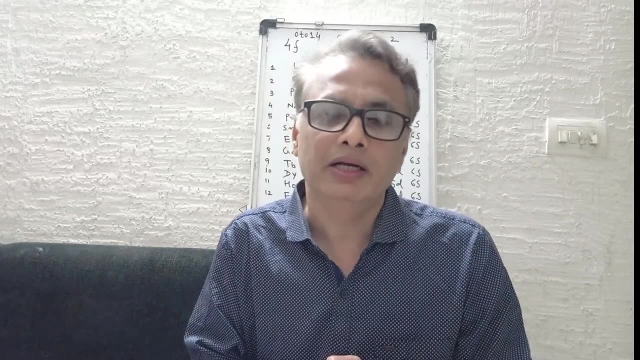 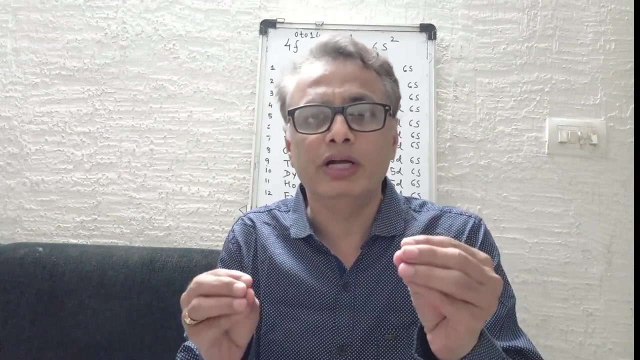 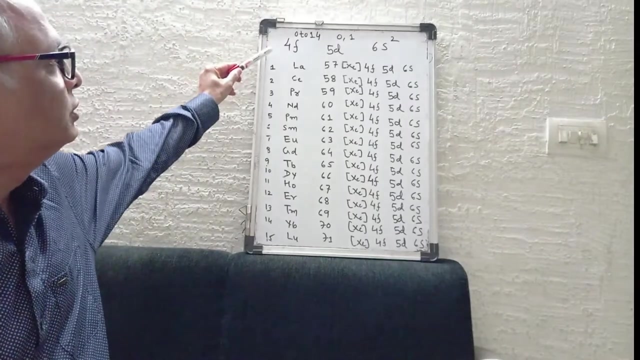 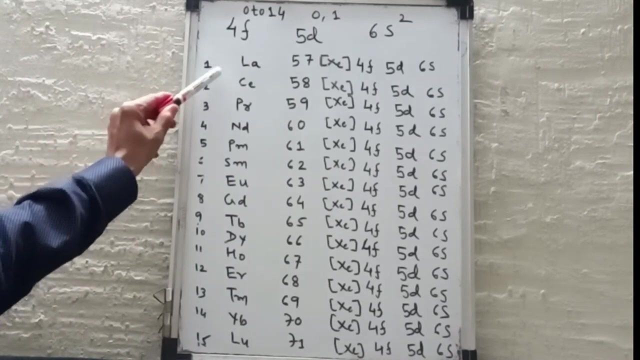 trick to remember: electronic configuration of lengthened element as well as name of the lengthened element element. so first of all we are going to write general electronic configuration of lengthen add element this way: 4s 0 to 40, 5b 0, 1, 6s, 2. here we are going to. 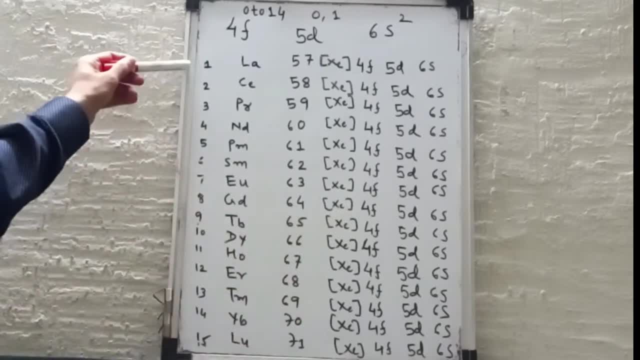 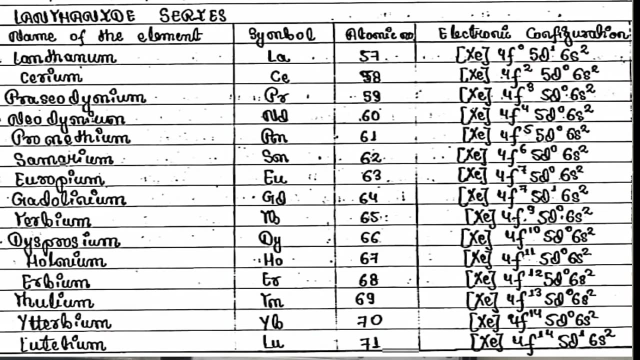 write 4 column. in the first column we are going to write number from 1 to 15. in second column, we are going to write name of the element. in third column, we are going to write symbol of lengthen add element. in fourth column, we are going to 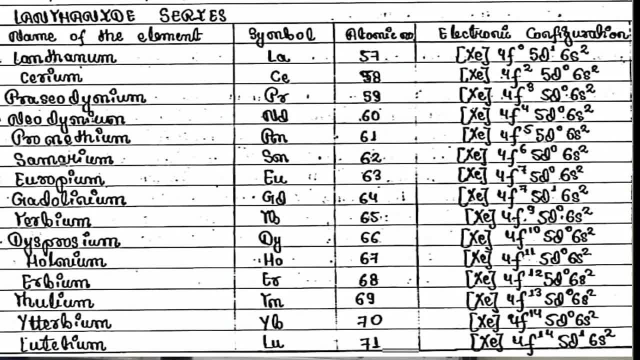 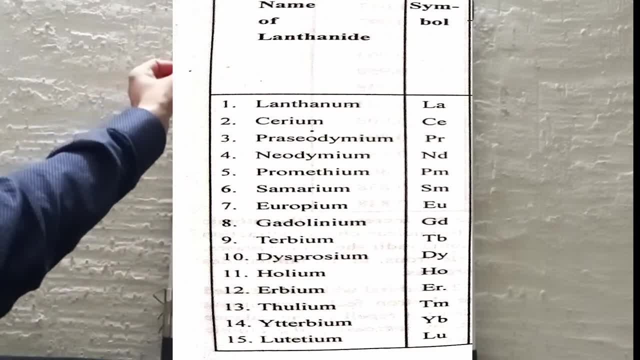 write atomic number and in fifth column we are going to write electronic configuration of lengthen add element. so first of all we are going to write all the lengthen add element, from lengthen up to lutetium. so we will write in this manner we like number, all the. 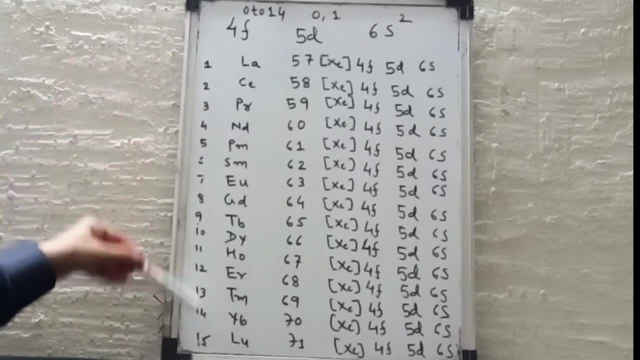 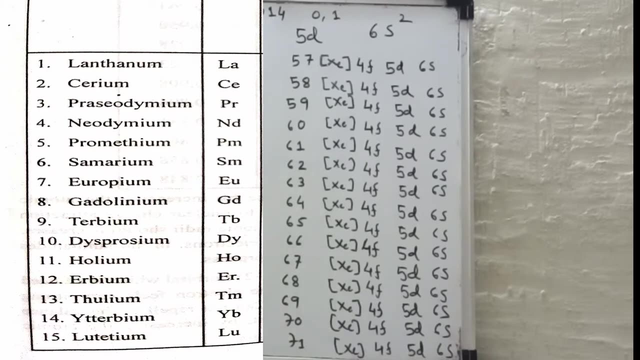 number in sequence from 1 to 15. first element of lengthen add series is lengthen up, hence it is known as lengthen add series. symbol is a, l, a atomic number is 57 and electronic configuration of is xenon: 4, f0, 5d1, 6s, 2. so in all this element, now I 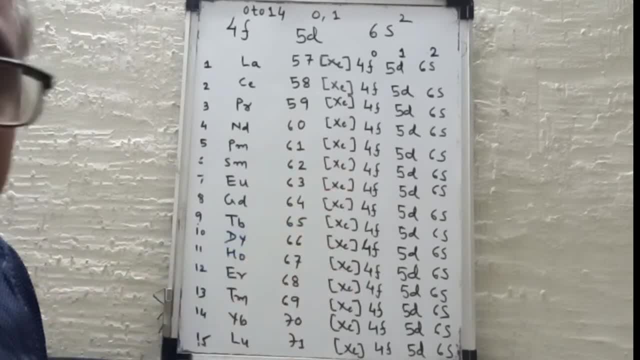 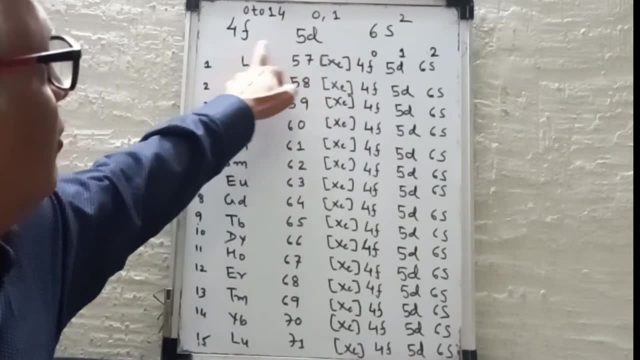 am going to give your trick to remember: electronic configuration of lengthen add. so this is general electronic configuration. so we would write for all this element 4f, 5d 6s in this manner: 4f 5d 6s for lanthanum cerium, pisodinium, neodymium. 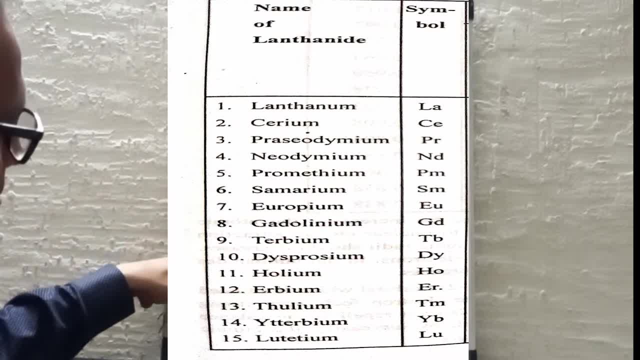 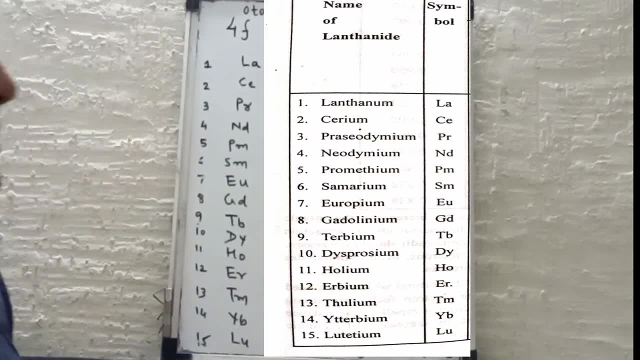 promethium, samarium, europium, gadolinium, carbium, dysprosium, holmium, erbium, thulium, ytterbium and lotatium. for all this element, we would write 4f, 5d, 6s in this manner. now what we'll do. 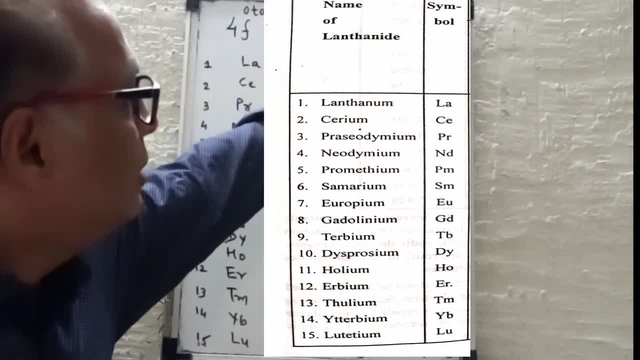 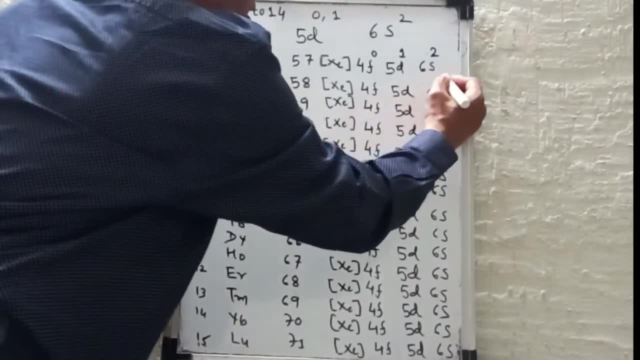 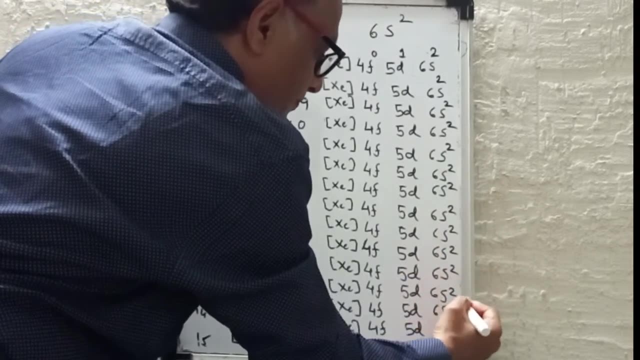 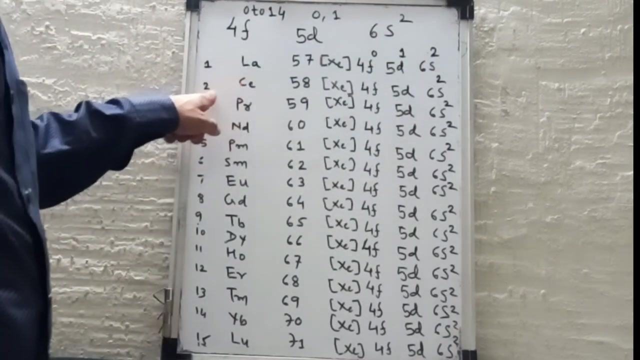 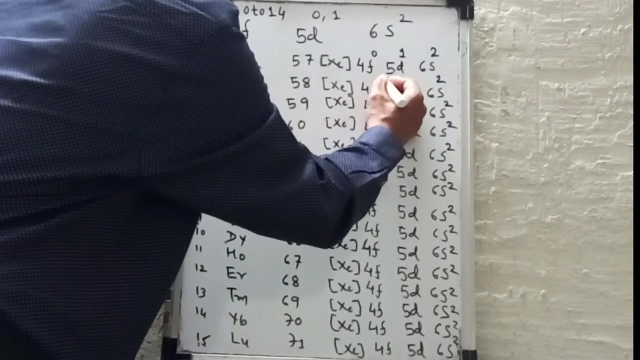 we'll write two electron in 6s orbital for all this element. so first here we will write two electron in 6s orbital. after writing two electron in 6s orbital, we will write two electron here. sequence is 2, so here we would write two electron in 4f. in third sequence we will write three. 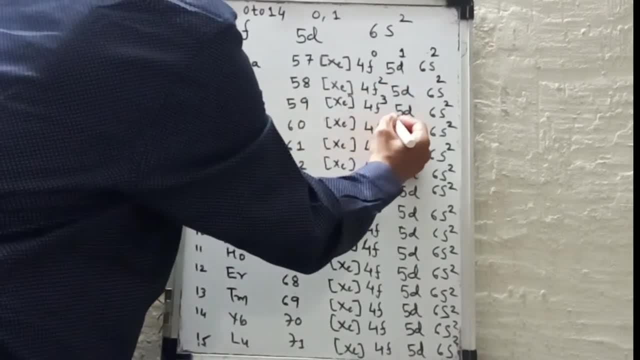 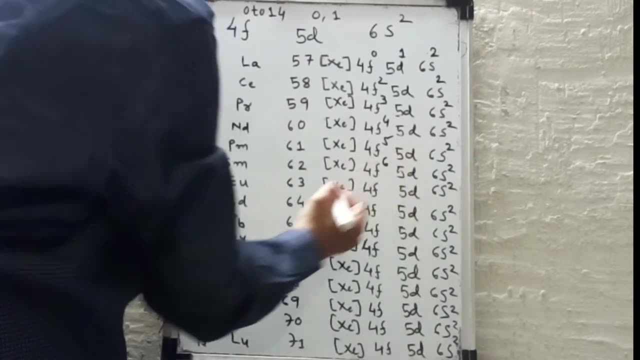 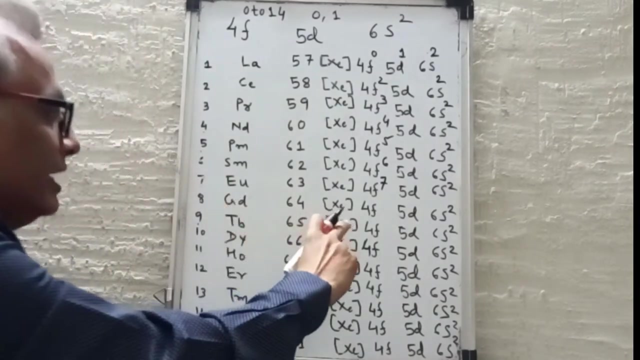 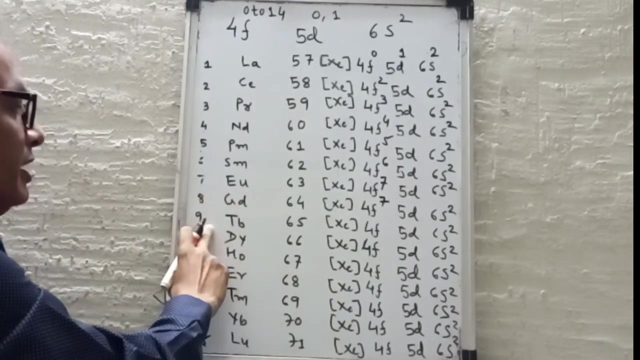 electron in pisodinium, four electron in neodymium, five electron in promethium, six electron in samarium, seven electron in europium. similarly for gadolinium we would write eight electron, but here we would discuss that, why we are writing seven in gadolinium. in therbium, we are going to. 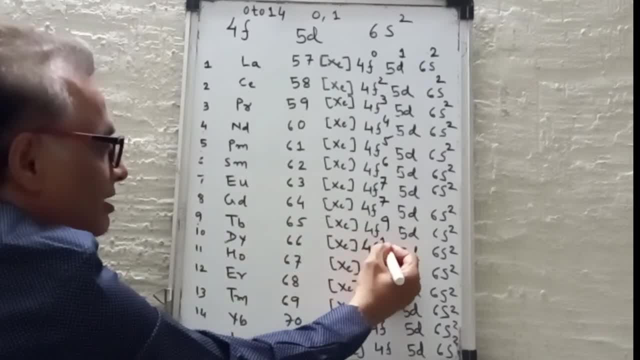 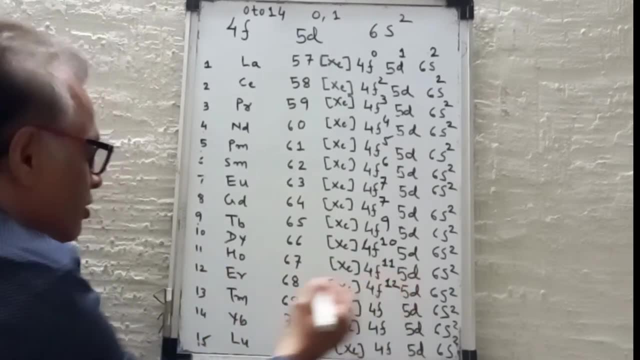 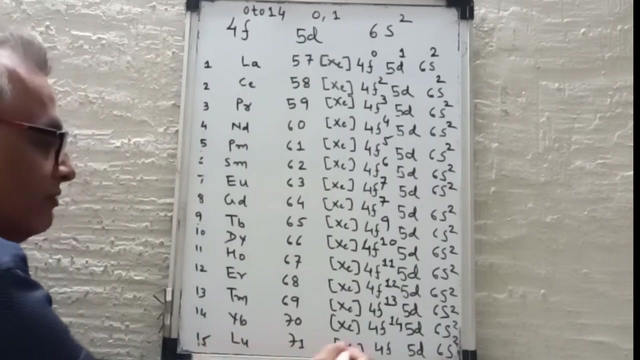 write nine, here we will write ten, here we will write eleven, and here we will write four. for holmium, for erbium, we would write twelve. for thulium, we would write thirteen. for ytterbium, we would write fourteen. here again we can write fifteen, but here, in order to gain stability. 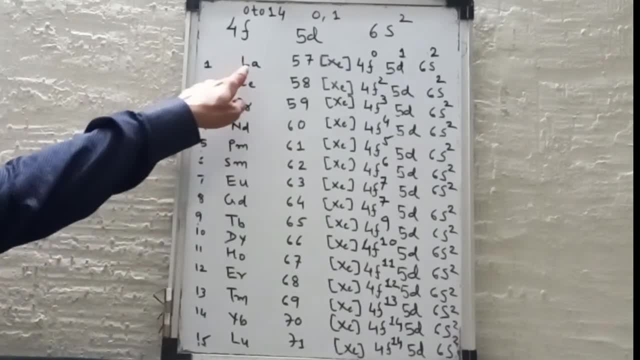 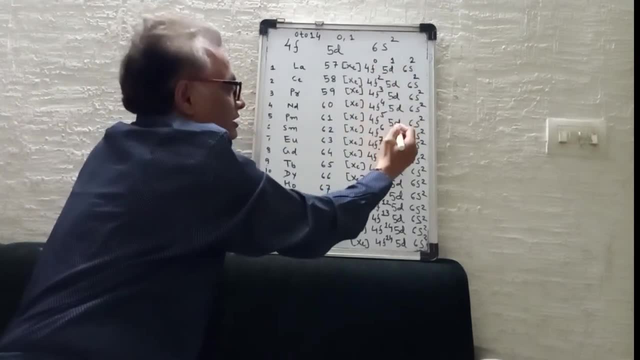 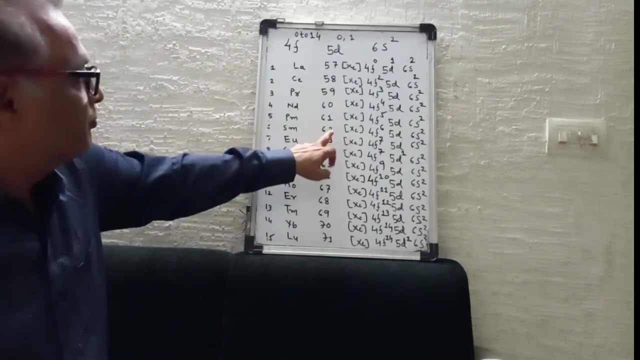 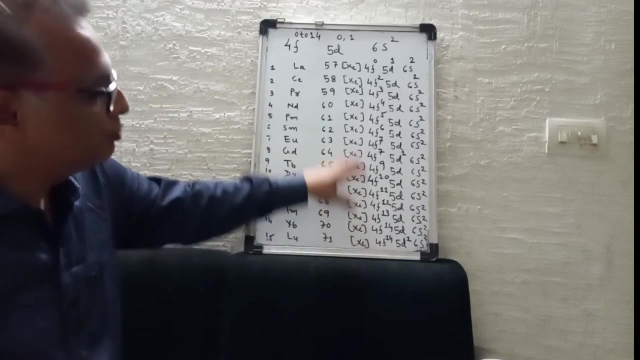 we would write fourteen. now for lanthenum, gadolinium and for lotatium we will write one electron in thagdy energy level. so So two times 4F7 will be repeated and two times 4F14 will be repeated. So this would be the electronic configuration of lengthened element. 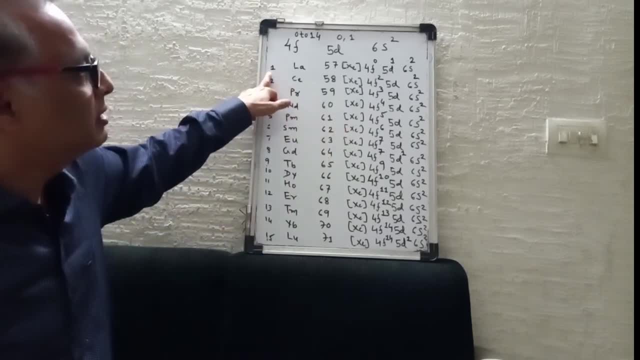 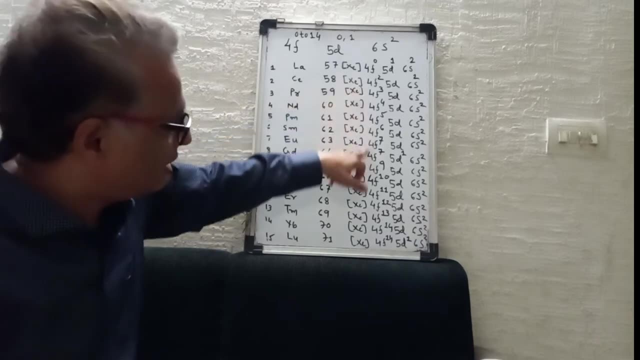 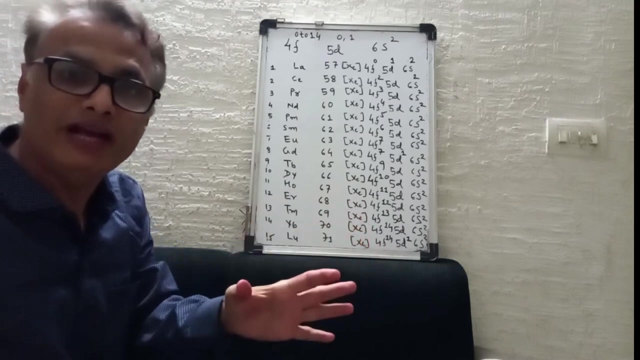 So, with the help of this trick, whatever the sequence number that you have to mention in 4F energy level, whatever the sequence number you have to mention in 4F energy level- okay, for gadolinium and lutetium, you have to write one electron in 5D energy level. you. 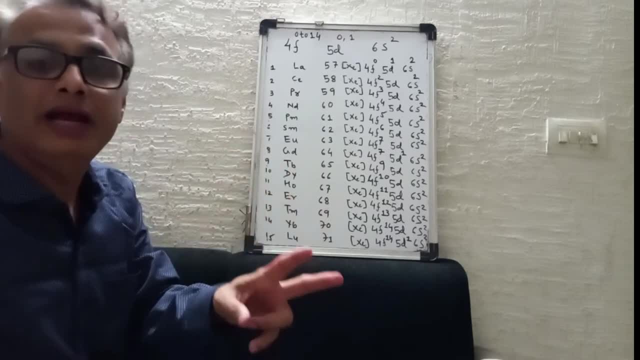 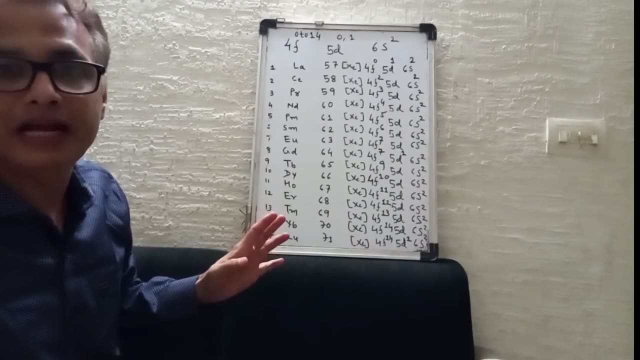 have to repeat two times 4F7 and two times 4F14,. okay, So in this way you can remember electronic configuration of lengthened element. Now how you are going to remember lengthened element. name of the lengthened element. 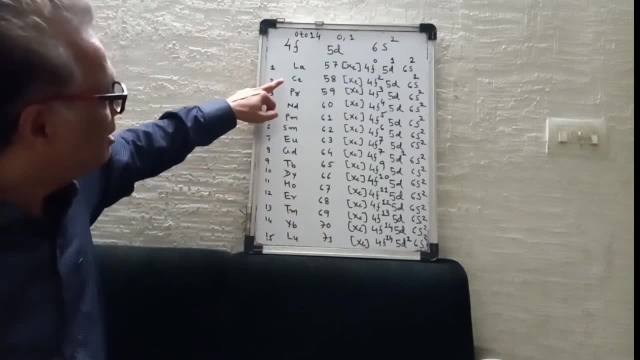 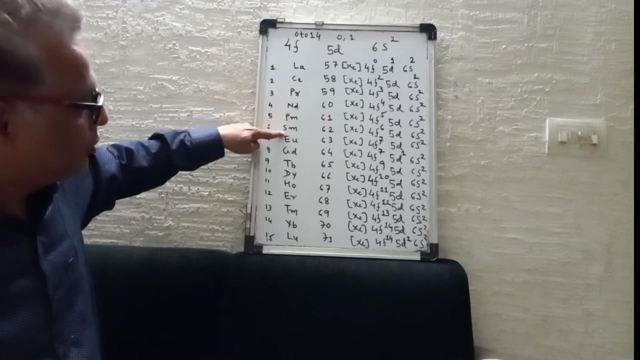 So, using this trick, you can remember all this lengthened element. You can, Because lengthened element starts from. So you can remember this way: Shriprasad nanth, shriprasad nanth, parivaar, samit yurog gaye tab daeria huwa or tu. 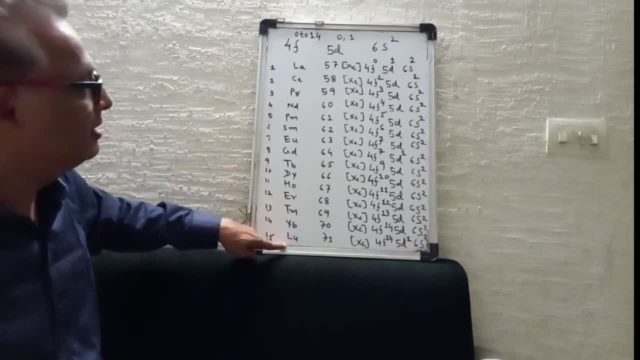 nyuhi lotaaye, Shriprasad nanth. parivaar samith yurog gaye tab daeria huwa, or tu nyuhi lotaaye, Shriprasad nanth. So hang on, I got it. 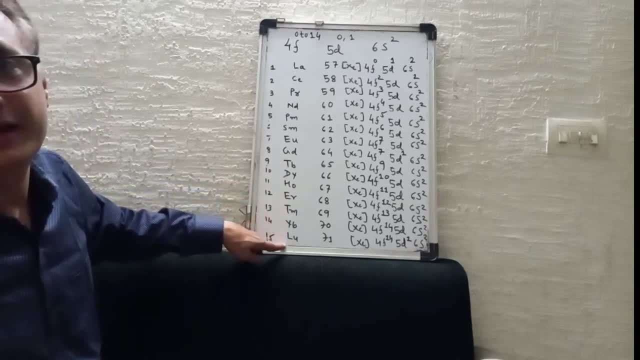 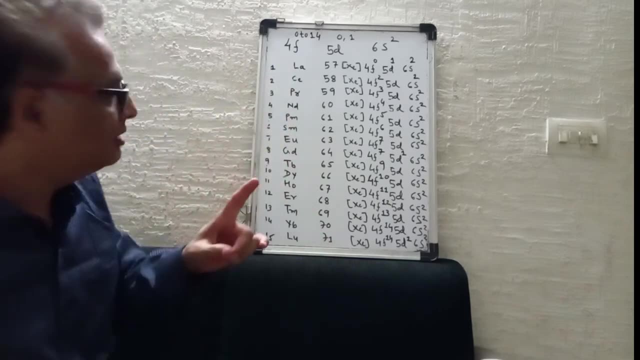 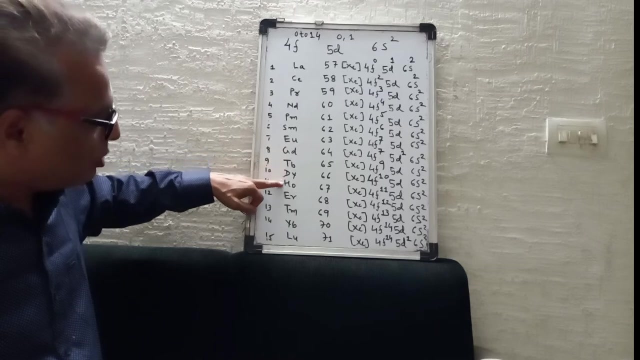 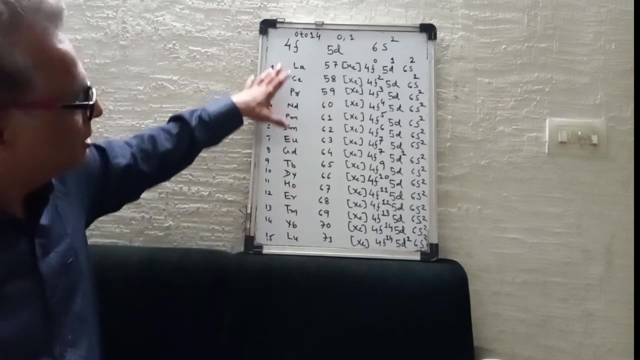 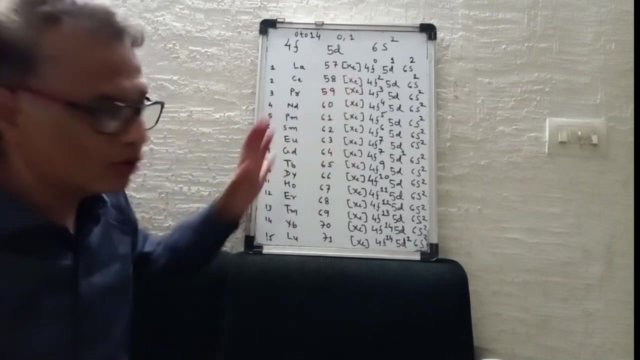 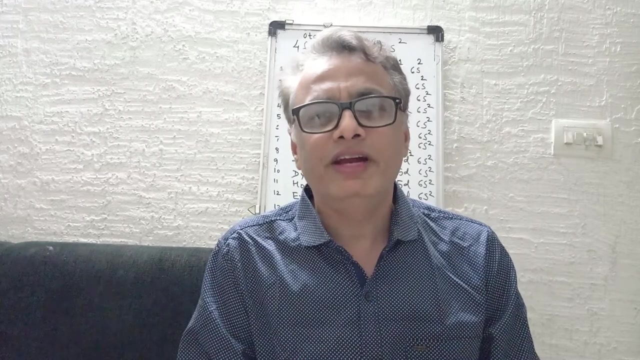 so, with the help of this trick, you can remember all the lengthen and element. I am repeating third time. so, with the help of this trick, you can remember name of the lengthen and as well as electronic configuration of lengthen and element. now, according to definition of lengthen and element, that the element in which new entering electron 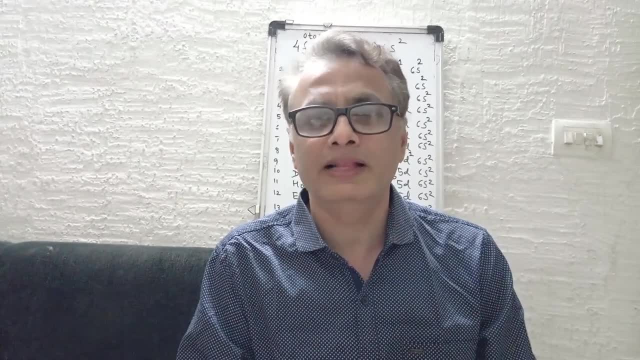 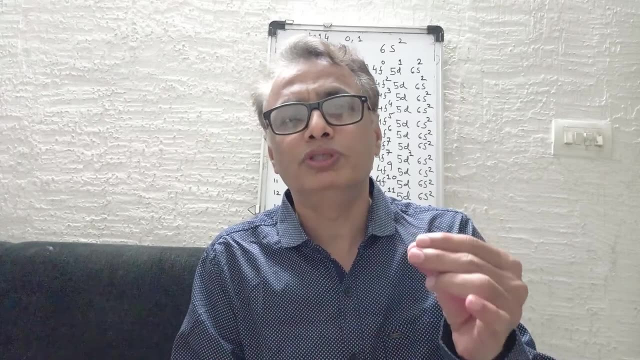 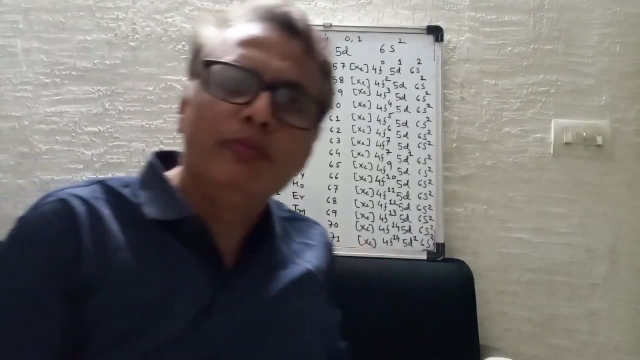 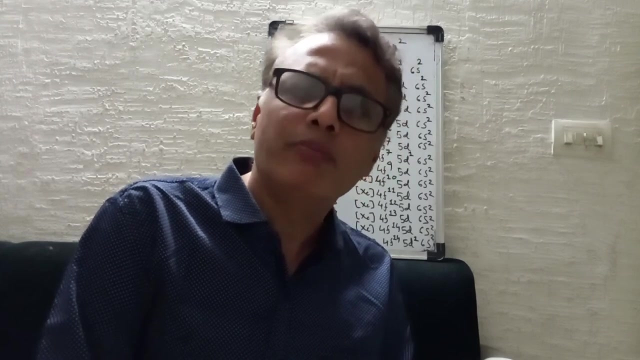 takes position in 4f energy level are known as a lengthen and element. according to definition, only 13 elements from cerium to ytterbium, atomic number 58 to 70, should be the member of lengthen and series. however, all the 15 elements from lengthen and to lutetium, atomic number 57 to 71 are considered as lengthen and element, since all the 15 elements have similar chemical and physical properties. generally, chemical properties depends on number of electron in outer energy level. in this element, new entering electron takes position in 4f energy level. so number of electron 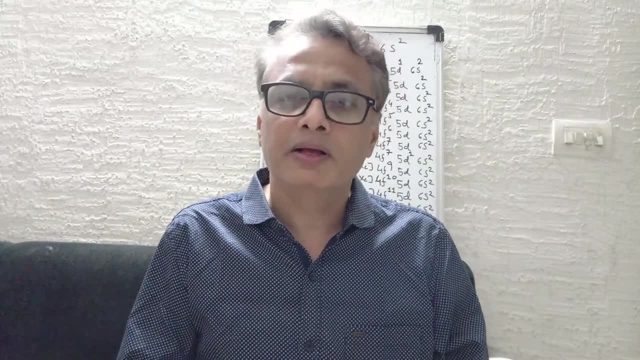 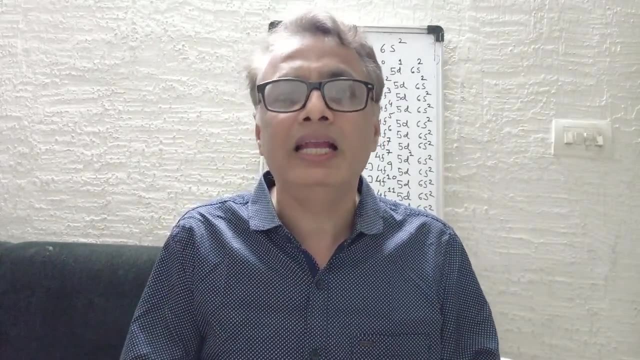 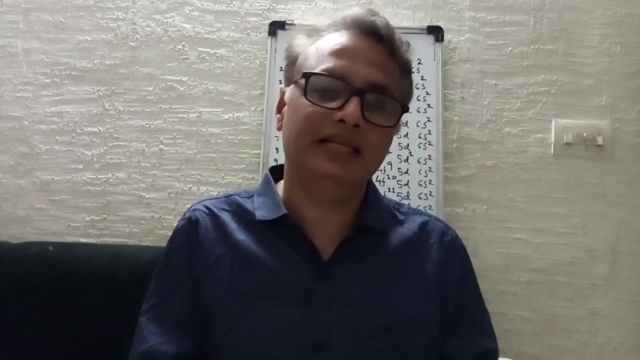 in energy level remains the same here. in lengthen and adapter, all the 14 elements are having similarity in chemical properties, and therefore lengthen and lutetium are included in lengthen and series. hodsetsthe number of struck by an equal mass of electronuties is equal to carrion charges. 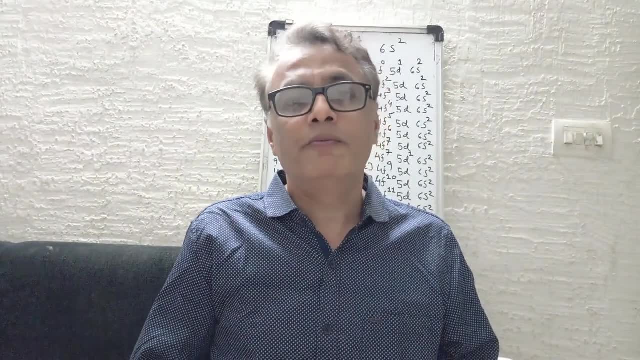 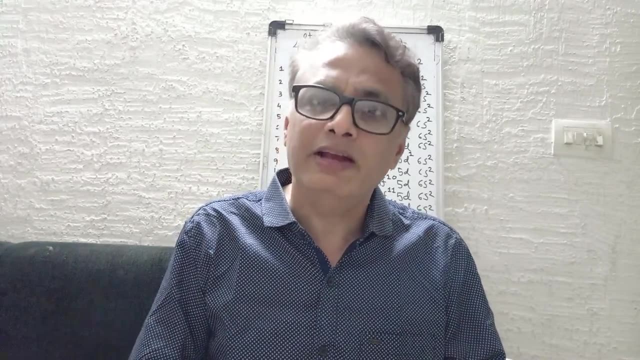 that wynn proud. these are all the 굉장히 sahaja. f intend Lência missing for a song. still she take this time to start a solamenteelf no longer on'the of gadolinium. electronic configuration should be from 4F8-5D0-6S2 instead of 4F7-5D1-6S2. 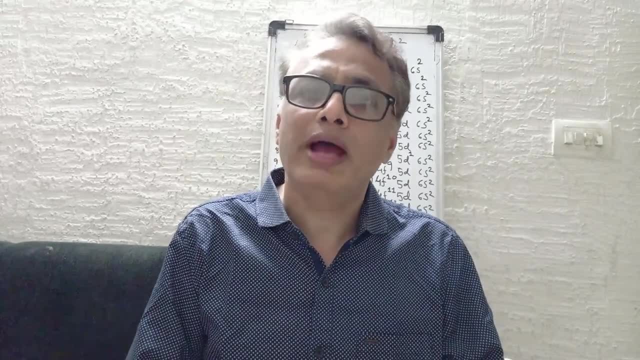 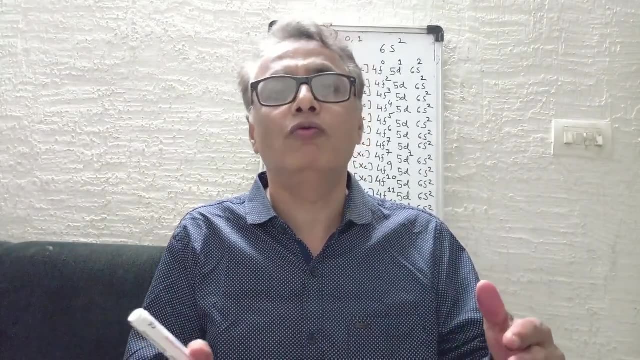 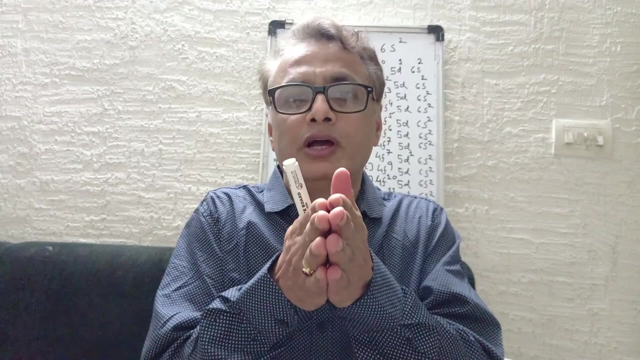 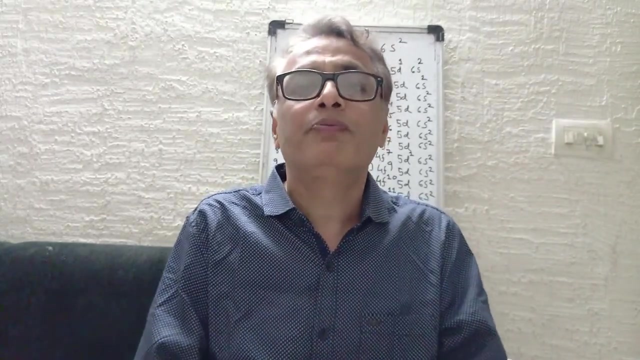 because in F orbital F0, F7 and F14 are stable electronic configuration and 4F8 it is quite near to 4F7 and energy difference between 4F and 5D is very close. difference between them is very less and therefore one electron from 4F transfer to 5D to give 4F7-5D1-6S2.